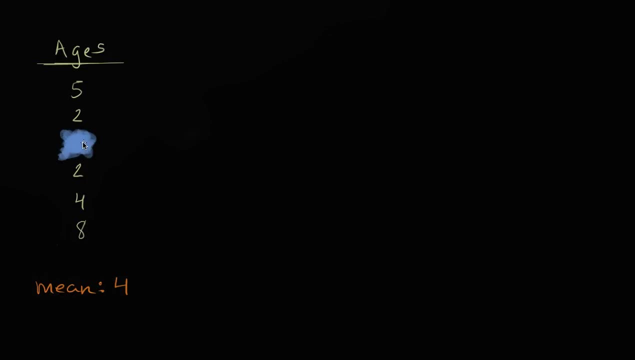 you notice that some blue ink spilled over one of the ages and you forgot how old that child is. And at first you're really worried. Your whole log system, your whole system of keeping records seems to you know you've lost information. 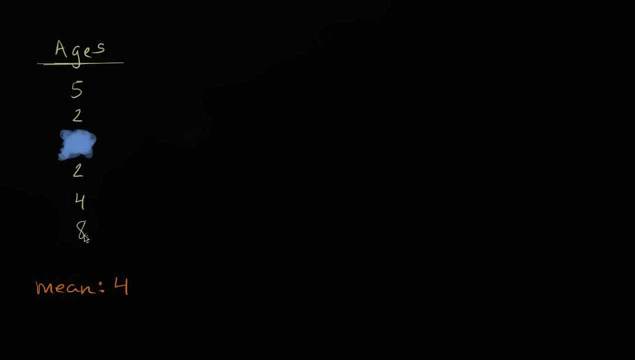 But then you remember that every time you wrote down a new age that month, you recalculated the mean, And so you have the mean here of being four. The mean age is four for the six children. So, given that, given that you know the mean, 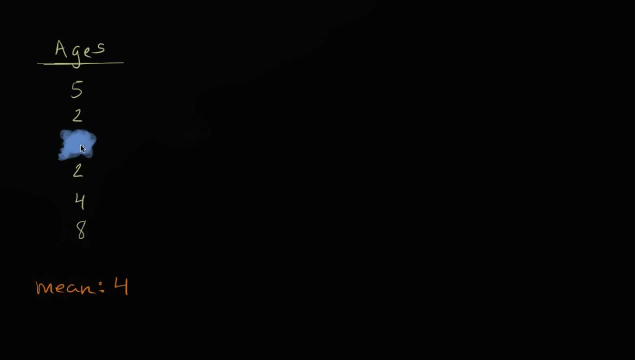 and that you know five out of six of the ages. can you figure out what the sixth age is? And I encourage you to pause the video and try to figure it out on your own. So I'm assuming you've had a shot at it. 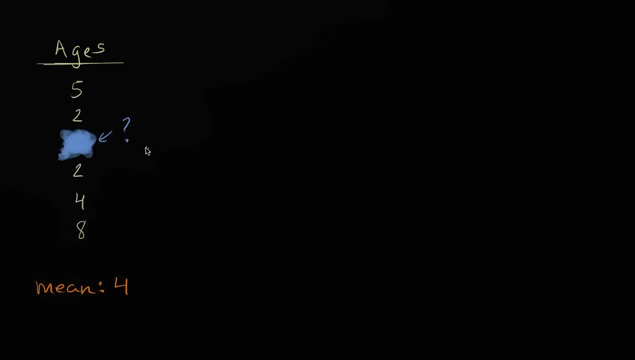 So let's just call this missing age, let's call that question, Okay, Question mark. So let's just think about: how do we calculate? how would we calculate a mean, if we knew what question mark is? Well, we would take the total. 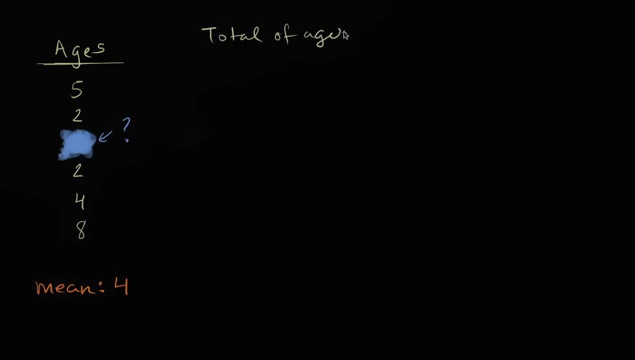 we would take the total of ages, of ages. We would then divide that by the number of children, We would then divide that by the number of ages that we had, And then that would be equal to. that would be equal to the mean. 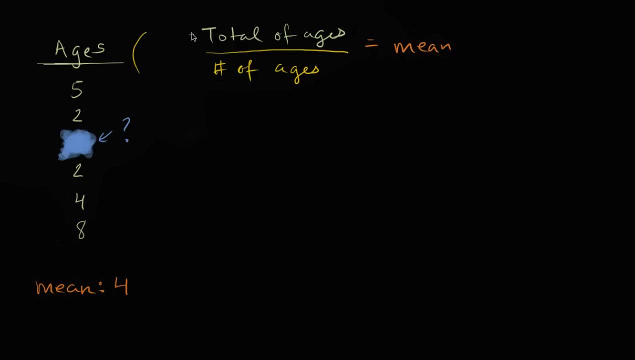 Or another way to think about it. if you multiply both sides times the number of ages- the number of ages on that side and the number of ages on that side- then this is going to cancel with that and we're going to be left with the total. 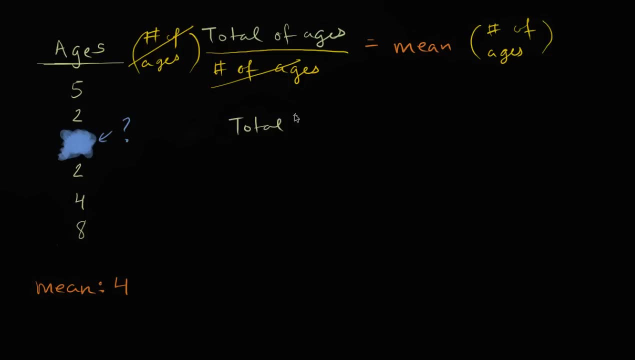 the total is going to be equal to is going to be equal to the mean times, the number of ages, Mean times, and I'll just write times, the number of ages, Number times, number of data points or number of ages. So maybe we can use this information. 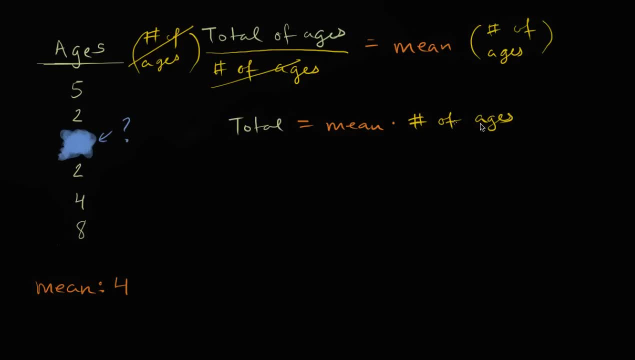 because we're just going to have this missing question mark here and we know the mean and we know the number of ages, So we just have to solve for the question mark. So let's do that. So let's go back to the beginning here. 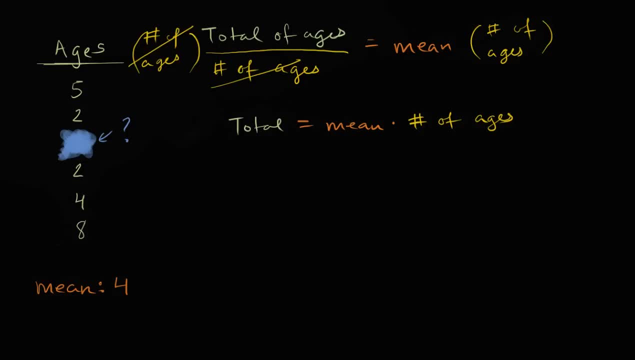 just so that this makes sense with some numbers: The total of ages that's going to be five plus two plus question mark plus question mark plus two. this two plus two plus four plus eight, We're going to divide by the number of ages. 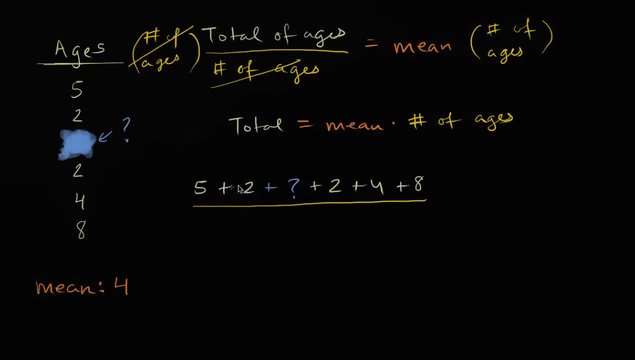 We're going to divide it by the number of ages. Well, we have six ages here: One, two, three, four, five, six, Six ages, and that's going to be equal to the mean. This is going to be equal to the mean. 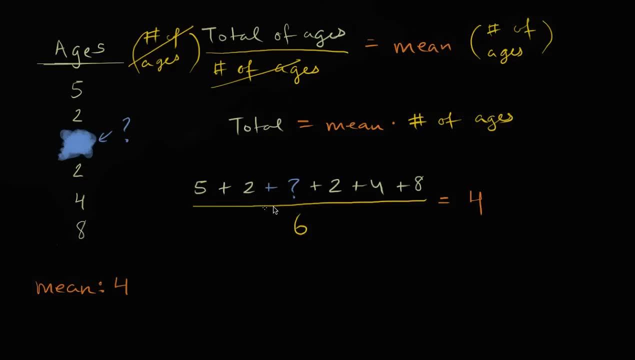 The mean here is four. So let's see, and this is just how you calculate the mean. So let's see how we, if we can simplify this. So five plus two is seven. Let me do this. that's the wrong color. 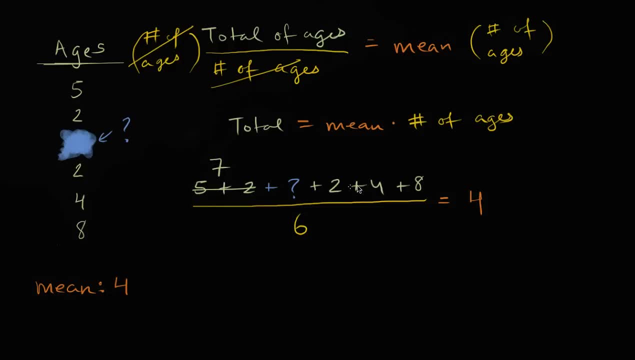 Five plus two. five plus two is seven, Two plus four is six. plus eight is 14,, 14.. And then seven plus 14 is 21.. So we're left with 21 plus question mark over six is equal to four. 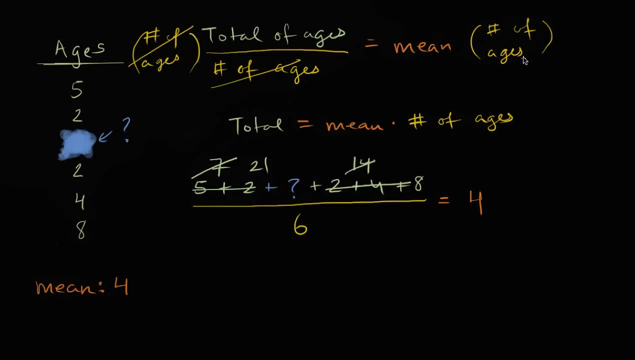 Now we can do what we did when we just wrote it all out: We can multiply both sides times the number of ages, the number of data points we have. So we can multiply both sides times six. We can multiply both sides times six. 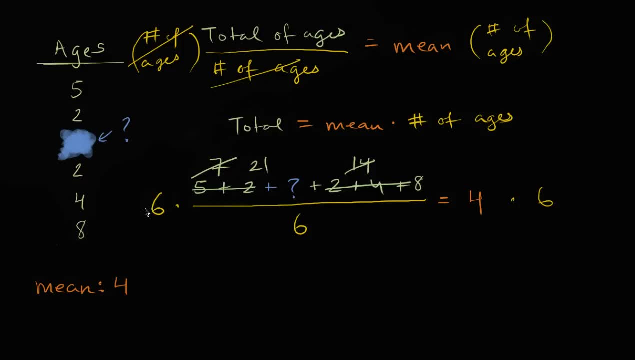 So six on that side, six on this side, Six in the numerator, six in the denominator. Those cancel. So all we're left is on the left hand side. we're left with 21 plus question mark right, All of these other green numbers. 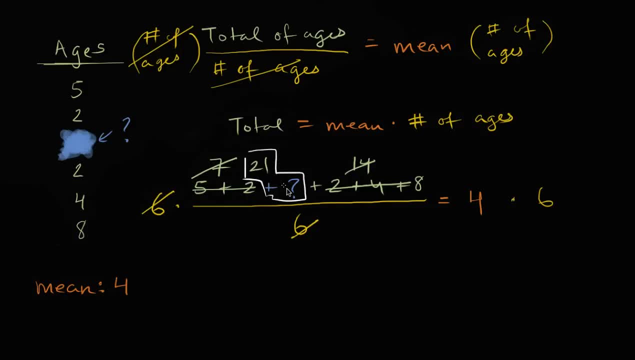 those are simple: five plus two plus two plus four plus eight is 21 and we still have the question mark. So we get 21.. Plus question mark. I want to do that green color: 21 plus this question mark, The thing that we're trying to solve for. 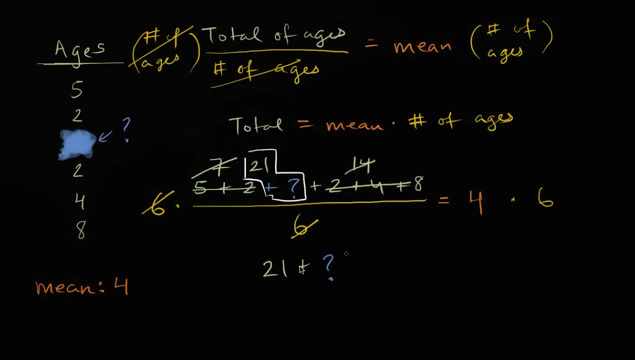 the missing number is going to be equal to is going to be equal to four times six. Well, what's four times six? That's 24.. And so what's the question mark? 21 plus what is equal to 24??